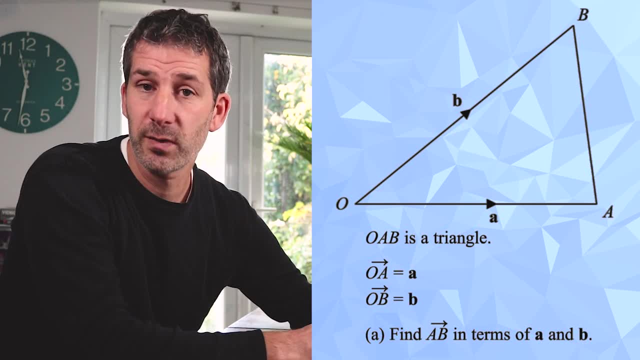 the vector that goes from A to B in terms of A and B, and the in terms of A and B is referring to that little a and little b written next to the triangle. They're written in bold there, but when we write them by hand, we instead we. 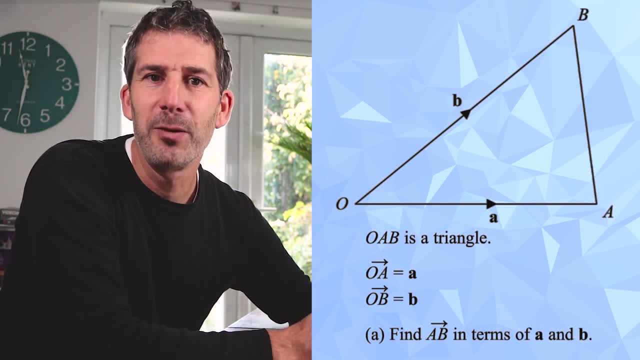 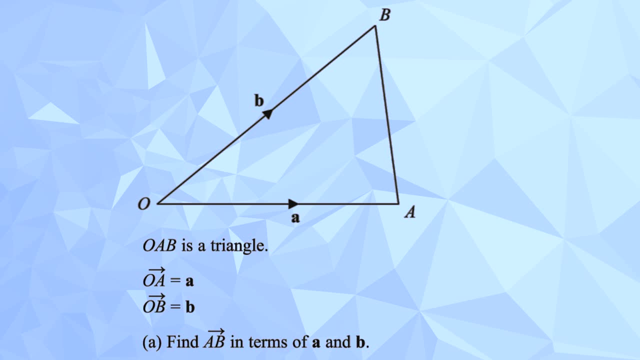 underline them well, because it is quite hard to write in bold. okay, So I use an analogy to help me make sense of vectors. It's not perfect, but it definitely helped me to get my head around the basic idea of what's going on, okay. 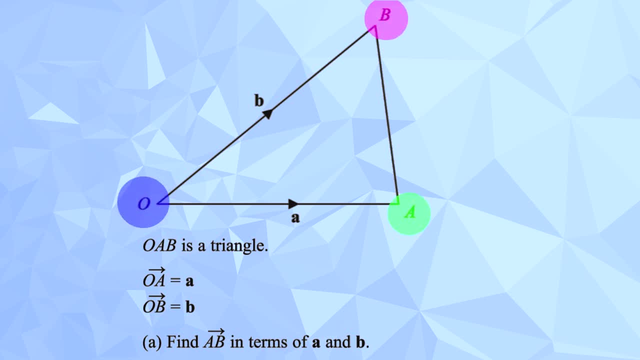 I think of A, B and O as three villages, and there's currently a railway that connects O to B and O to A. The fact they have the little letters A and B next to them, that tells us that there's a railway line there. okay, So the journey. 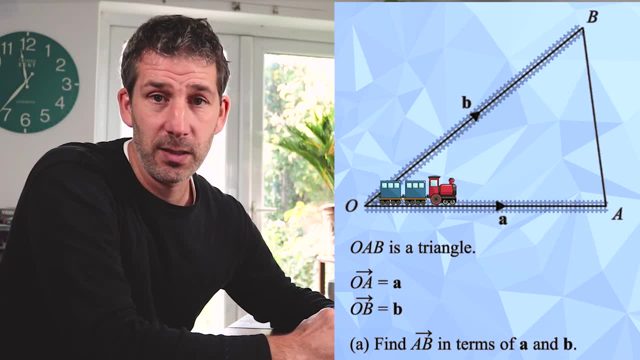 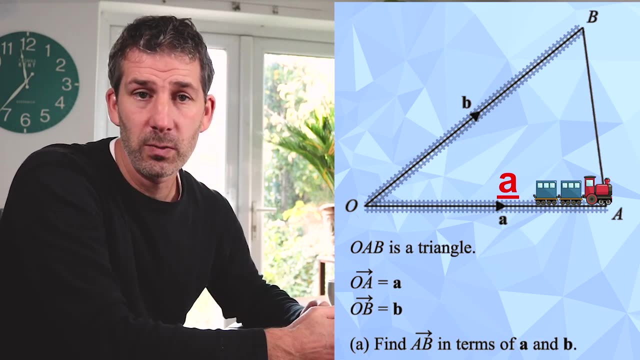 that the train makes from O to A, we call that vector. A okay, and a vector is really just a journey. and if we want to go in the opposite direction, from A to O- we call that journey negative A And that little arrow you can see that lets you know the direction of the. 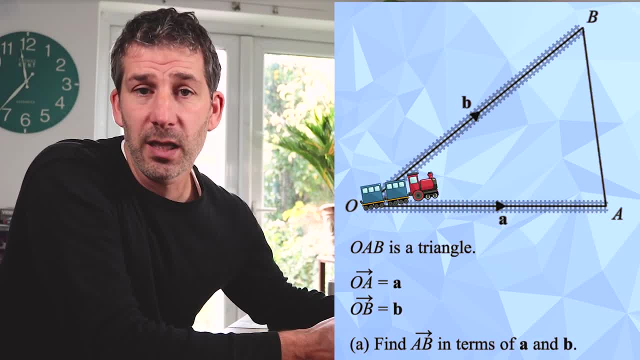 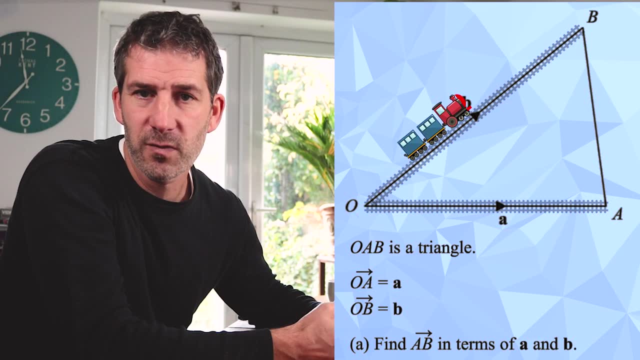 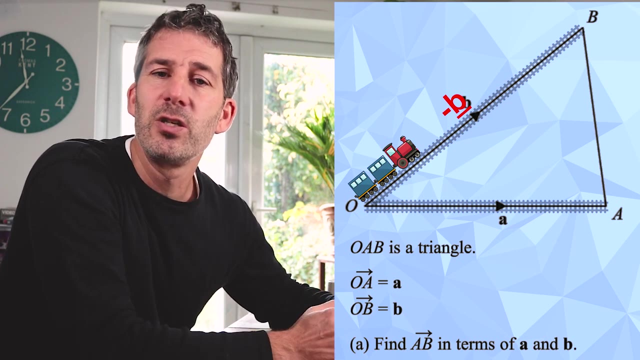 journey. okay, The journey from O to B, then, is called vector B, and to come back in the opposite direction to the way the arrow is pointing, in other words from B to O, we call that vector negative B. So to come back in the opposite direction, you just make the letter negative. Now the 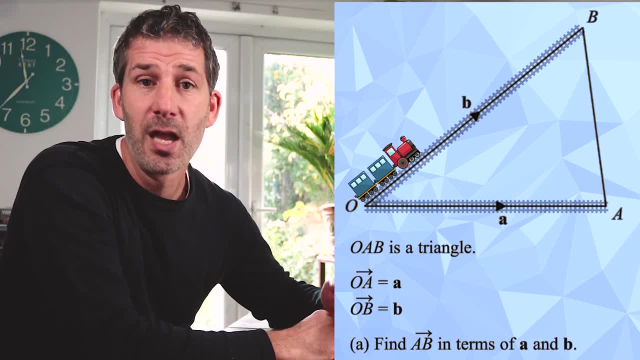 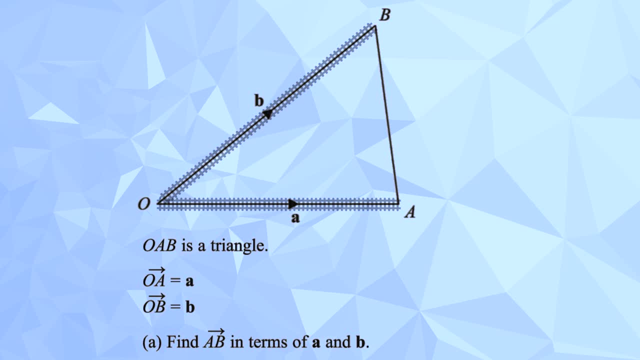 question is asking us to find the vector that goes from A to B, but at the moment there isn't a train line that takes us directly from A to B. There is a line on a diagram connecting A and B, but it doesn't have a little letter next to. 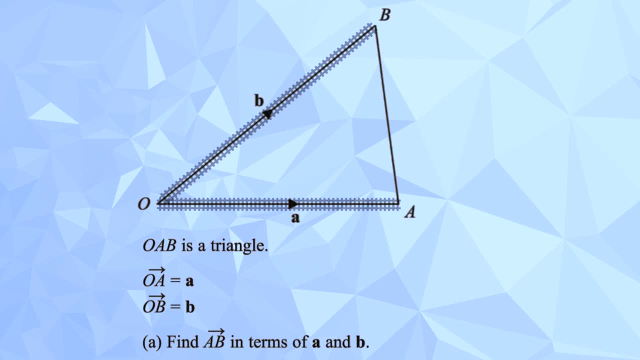 it. so currently there's no train journey that takes us from A to B, But we can make that journey using the train lines that we do have. All we need to do is to go from A to O- and we know that that's called negative A- and then from O to B. 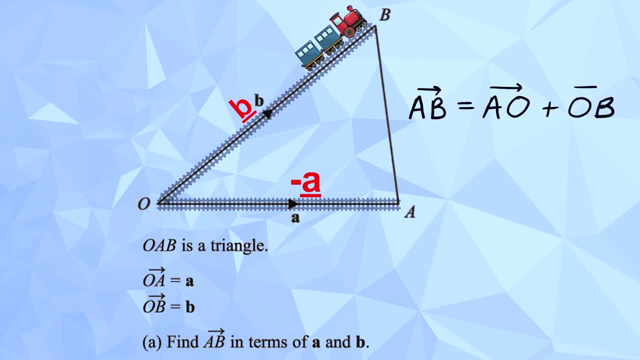 and that's vector B. So we could describe the vector A to B as negative A add B. I'm going to go through a second example before we move on to look at the midpoint of lines. I'll put it up on the screen for a few seconds, so pause the. 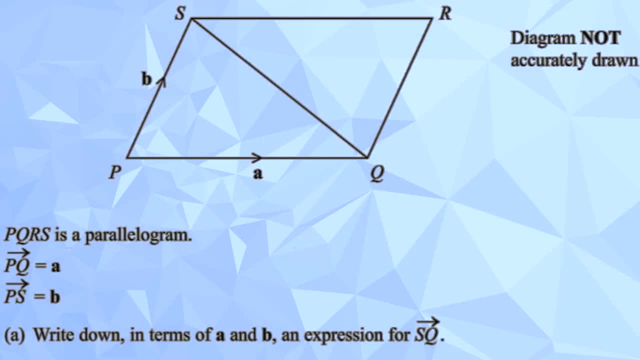 video and have a go yourself, and then I'll be back in a moment to talk you through it. So I hope you are able to do that. don't worry if not. I'm going to go through it now Before I do that. if this is your first time at the channel, welcome. it's very. 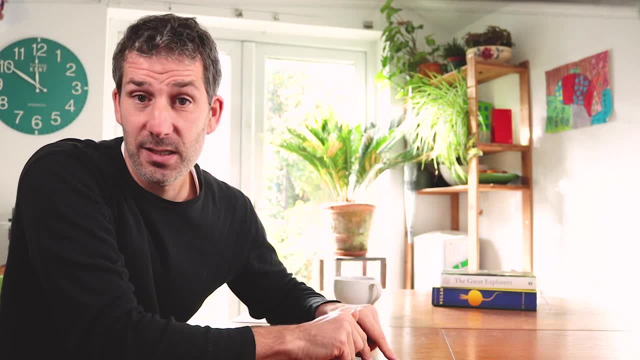 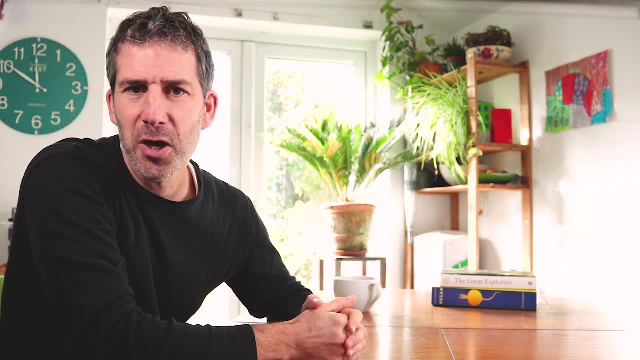 good to have you here. I put up full-length videos like this every Thursday and I do shorter tips and tricks style videos every Monday. I'll leave some links at the end of the video if you want to have a look at some of those other ones that I've done. Also, if you found the video helpful, it really 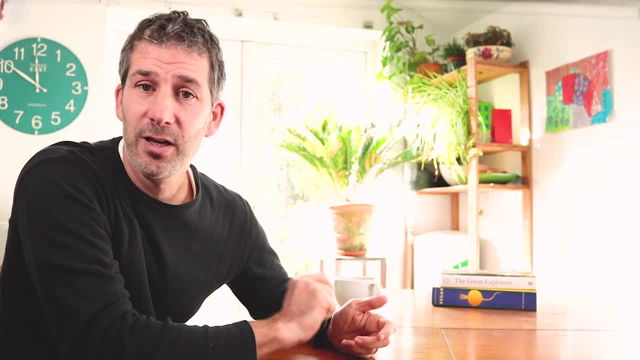 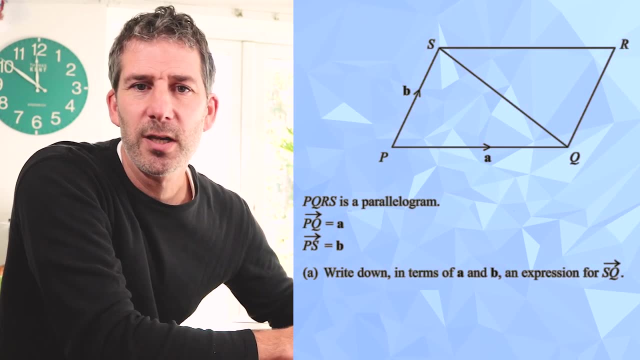 helps the channel to grow and to become successful if you give it a little like or even consider subscribing if you haven't already done so. Right back to the question. So we're being asked to write, in terms of a and b, an expression for vector sq. 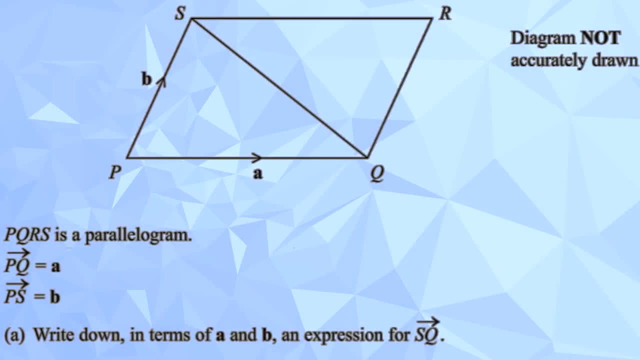 Rod, how do you think we can do that? Looking at this, it's a lot different to the one before, so I guess it would be minus b plus a. Yeah, yes, yeah, yeah, yeah. so how come? Well, it's got to go from s to p to q, so it's s going backwards from b, so that's minus b, and then it's going forwards to s. 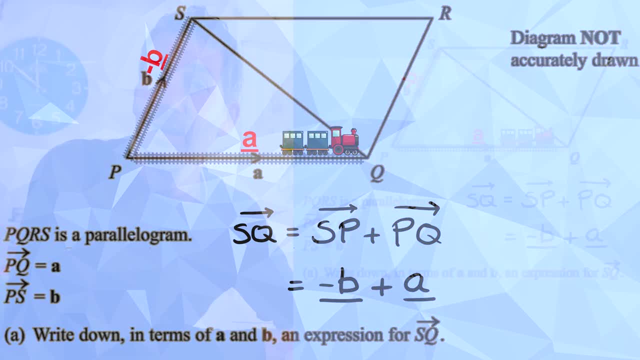 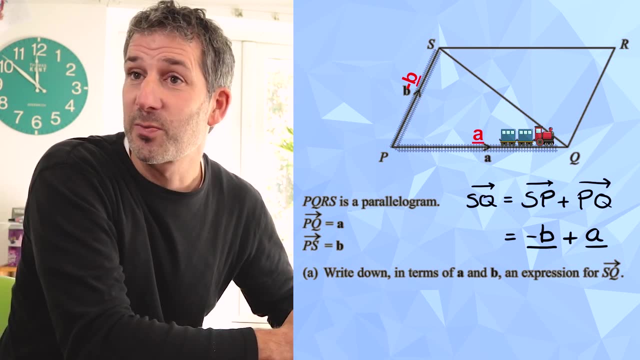 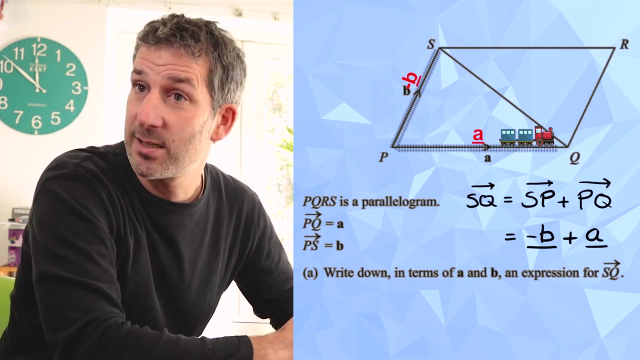 It looks like a different shape, doesn't it? Well, it is a different shape, but actually, within that, it's really just the same as the previous one, isn't it? It initially looks different, but actually it's basically just the same thing, So don't let that. yeah, yeah, exactly. yeah. just look at kind of half of it. 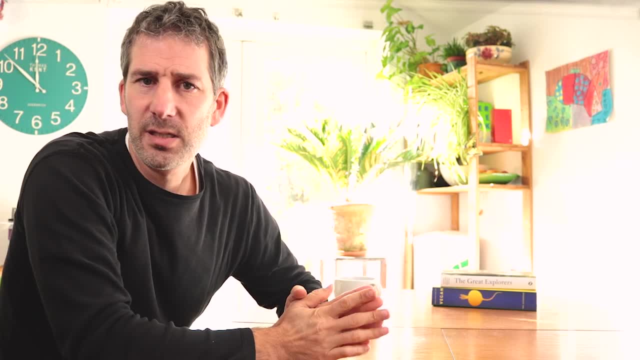 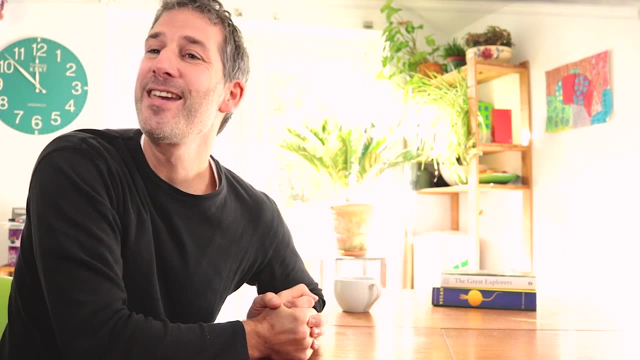 Brilliant good. thank you Right now. so the second part of the video. we're going to look at the questions that involve midpoints. Rod, what do we mean? What do we mean by the word midpoint? The middle of a point, Right exactly at the middle of that line? yeah, 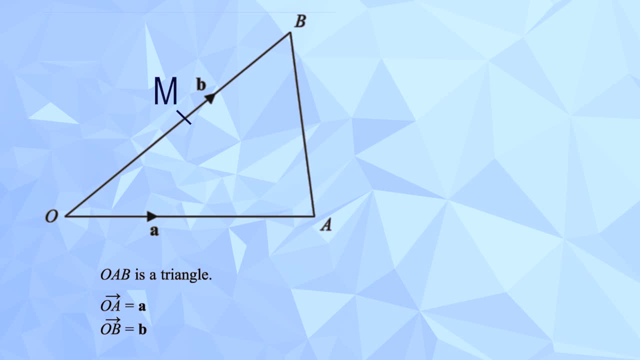 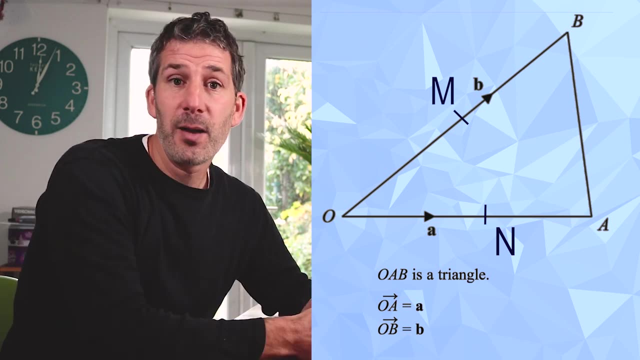 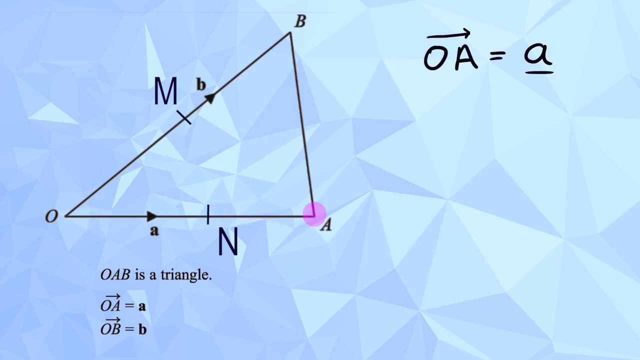 Let's go back to our original question. Let's say we were told that m is the midpoint of ob and n is the midpoint of oa. That just means that m and n are both exactly halfway along those lines. okay, So if o to a can be described as vector a, then o to n is half of them. 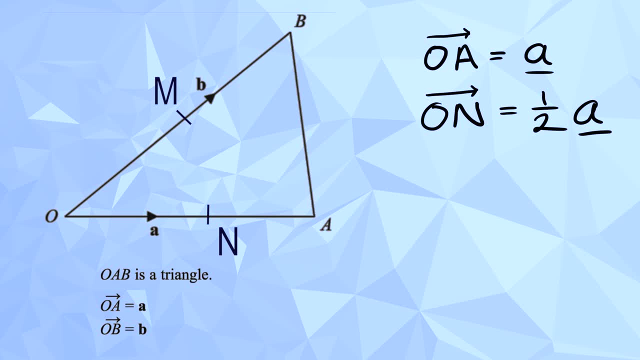 We would just say it's half a. Vector b to a. Vector m is half of bo, and we know that bo is negative b, so vector bm is negative half b. okay, But what if we were given the midpoint of a to b? okay. 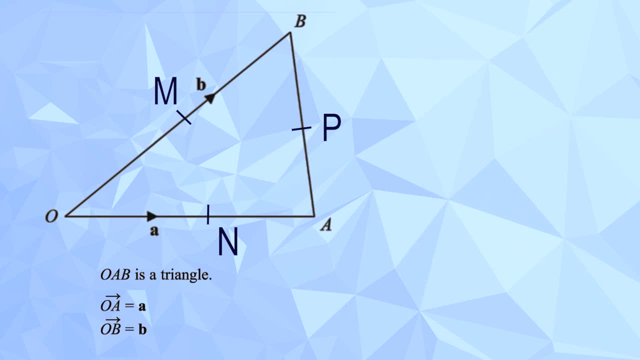 We'll call that point p. How would we describe the vector ap? Well, ap is just half of ab, so all we have to do is find ab and then half it. okay, And we actually worked out ab earlier on. So negative a, add b. 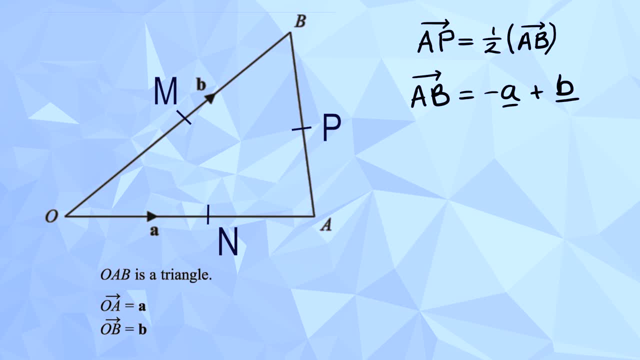 So ap is half of that and you have options as to how you're going to write that. You could say negative a, add b over 2 or divided by 2.. You could use brackets to show that you're multiplying both of those by a half. 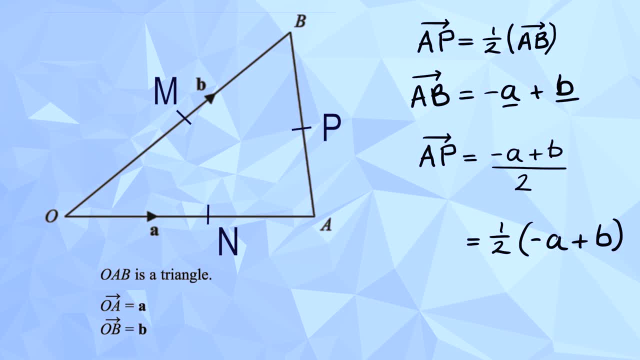 Or in other words, that you're halving each of them, Or you could kind of expand those brackets. Essentially, you could just half each of those. okay, So, negative: half a add half b. right, All of those mean the same thing and they're useful in different situations. 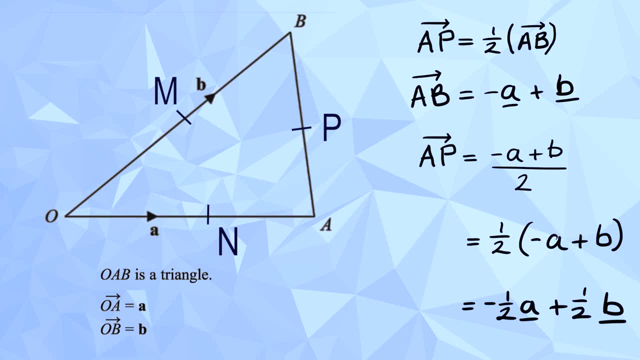 It depends what you're working out and what stage of the working out you're at, But the simplest way to describe it here, I think anyway, is negative: half a add b, So we'll go with that, okay. Well, what if we were asked to describe the vector op? 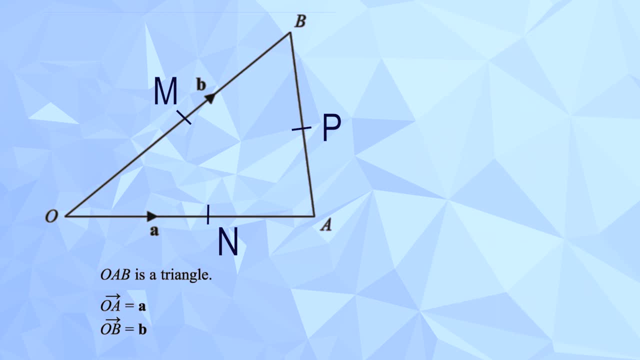 Well, to go from o to p, you could go from o to a And then from a to p, And we would write that like this: Now we know that o to a- we just call that vector a- And from a to p. well, we just worked that out. 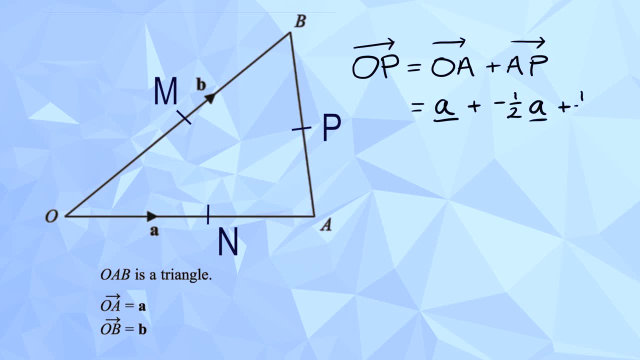 It was negative half a add half b. So if we put that together, we've got a add negative, half a add half b, And we can simplify that a bit. So the a add negative half a. Well, if you're adding a negative half a, that's really just the same as taking away half a. 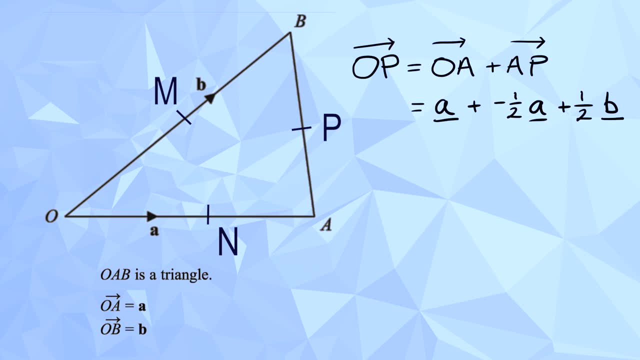 So we've got a minus half a and then add half b. Well, a minus half a, that's just half a. So we end up with half a add half b. We're virtually done now. actually, I want to give you one more question to practice. 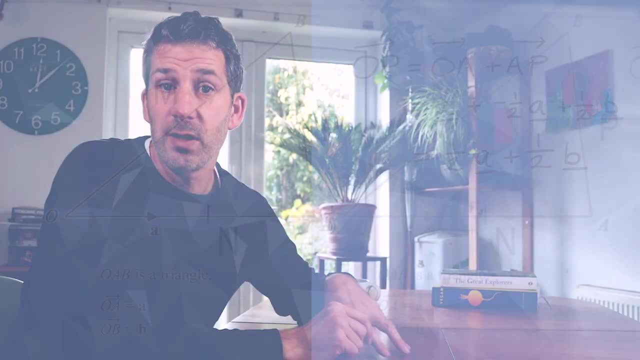 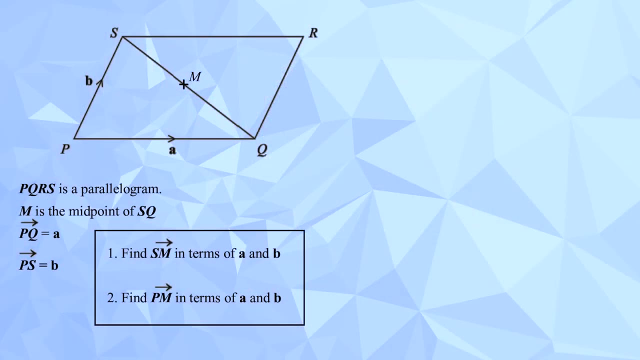 And in fact, it will be a continuation of the one you did earlier And we'll come back in a moment to go through the answer. So, as usual, pause the video, Have a go yourself. Okay, how did you get on with that? I hope it was okay. 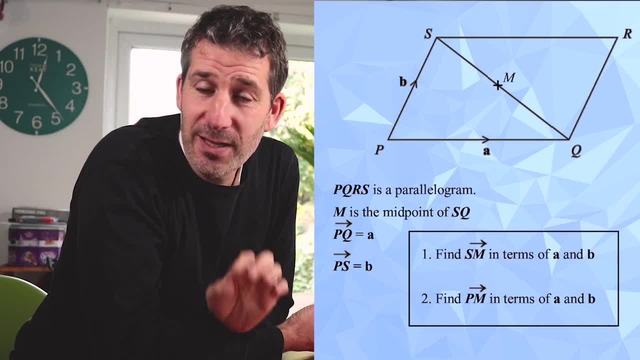 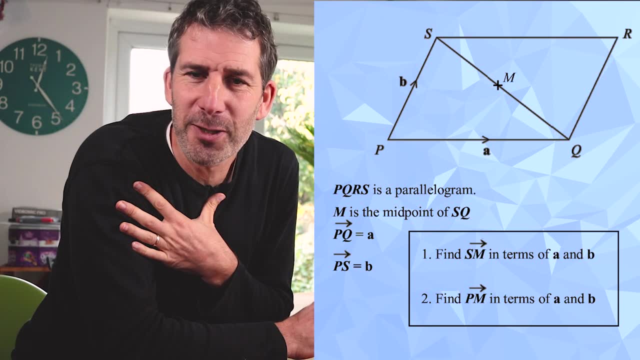 But don't worry if it wasn't. This is quite a difficult subject And it definitely takes a little while to get used to. So we'll talk through that question now. We'll see how you did compared with us. Rod, talk me through it. 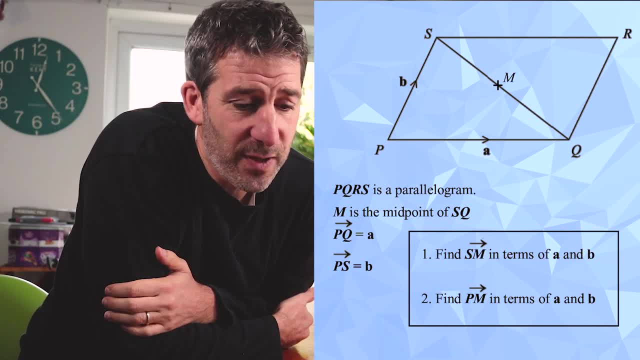 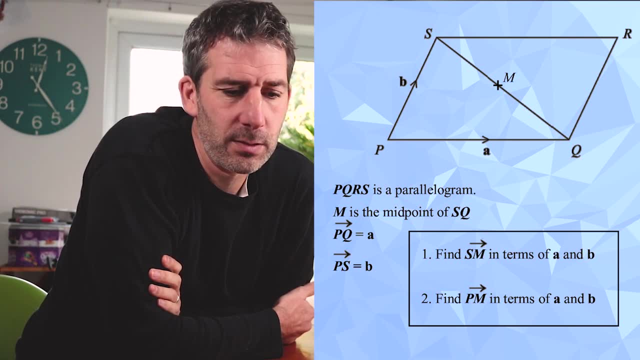 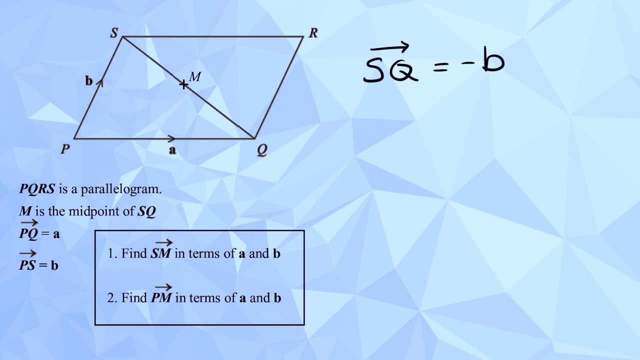 So the first bit, we were being asked to find the vector sm, To describe the vector sm. So to find the half you need to go to s to q, So it would be negative b to positive a. Can I pause you there? You're absolutely right. 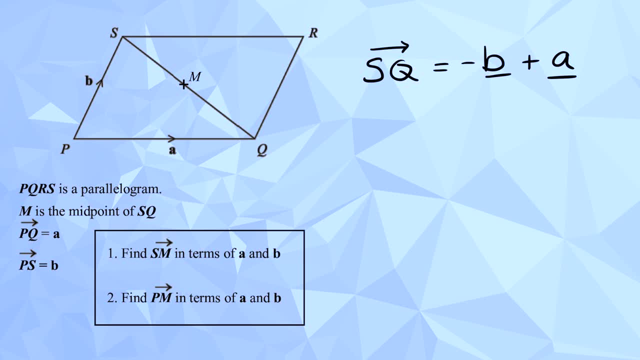 So to find sm. What you're saying is, before we can do that, We've got to work out that vector s to q. Yeah, Absolutely right. So you said that was negative. b add a. Yeah, Perfect, I agree with that. 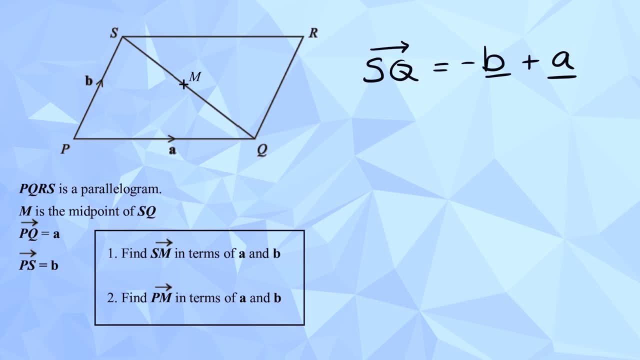 Spot on Good Right, Because m is half way through Right, Then it's half of that. So it would be negative half b plus half a. That's perfect. So s to m is exactly half of s to q, So it's just going to be half of what we got for that bit. 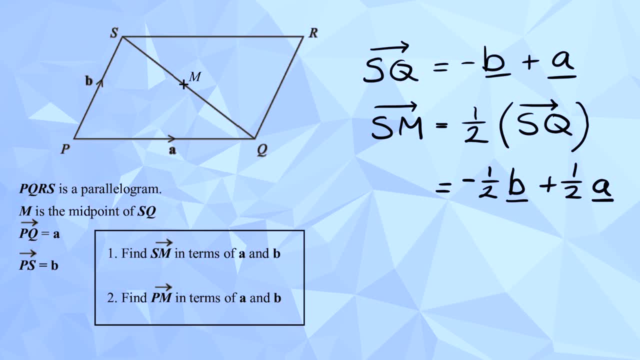 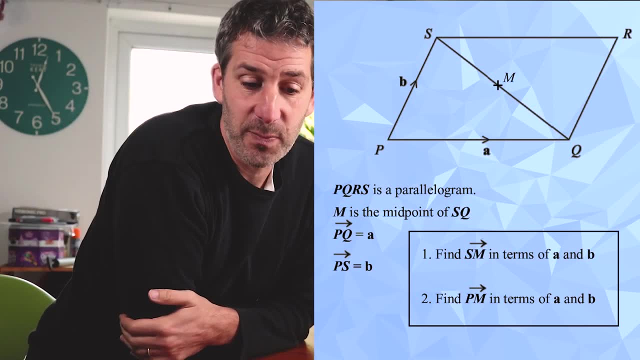 So yeah, You're absolutely right. Negative half b add half a. Brilliant, Good man, Good man, Right. And what's the second bit? To find pm, Vector pm, Or from p to m, P to m. So the easiest way would be to go from p to s. 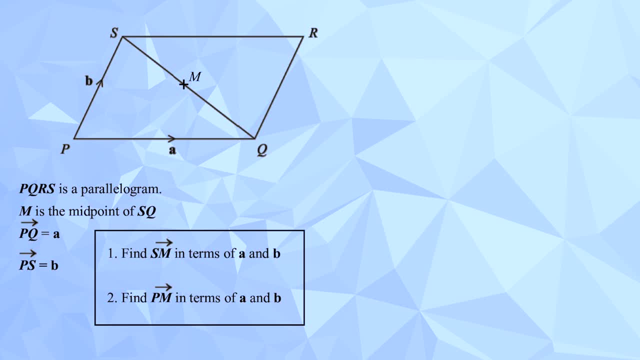